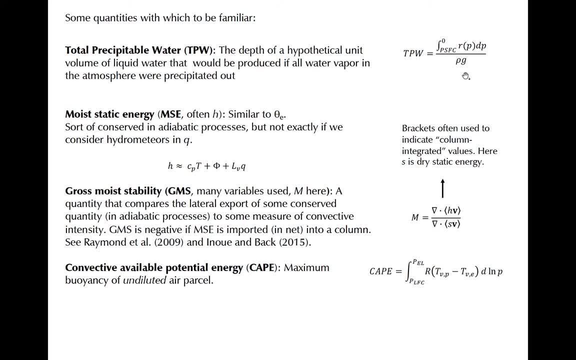 millimeters correspond to values of column relative humidity that are sufficient for widespread deep convection. Moist static energy is similar to theta E. It is approximately conserved in adiabatic processes. It is the moist enthalpy- these two terms- and the moisture density. these two terms are: 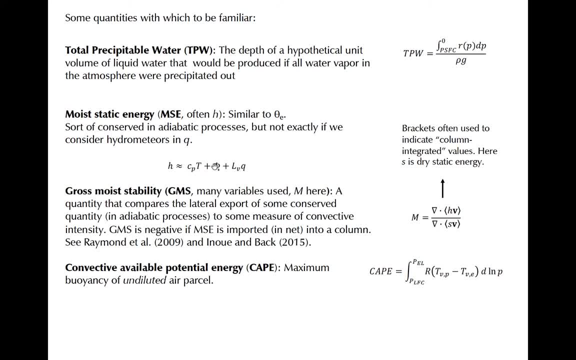 the two terms plus the geopotential. The gross moist stability is a metric that is sometimes used to assess the large-scale thermodynamic support for widespread deep convection. If GMS is negative, the environment is considered unstable. We won't see GMS on a skew T diagram, but it is a useful concept that will come up. 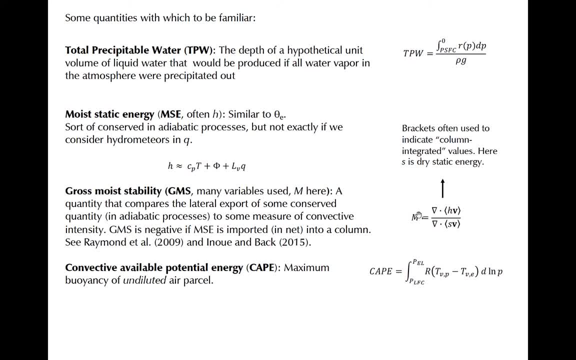 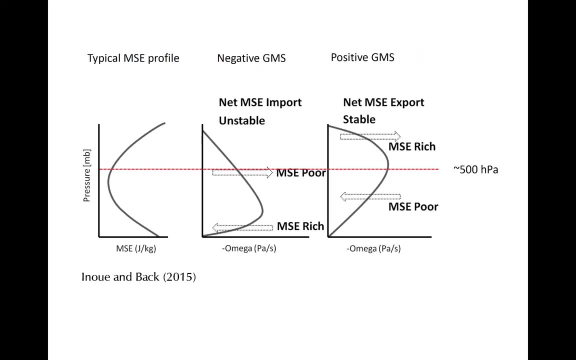 again later in the course and I bring it up now because of its relationship to the MSE profile which is indicated in the equation here. A typical MSE profile in the tropics is seen at left. It looks like the theta E profile seen before and it has a minimum somewhere in the middle. 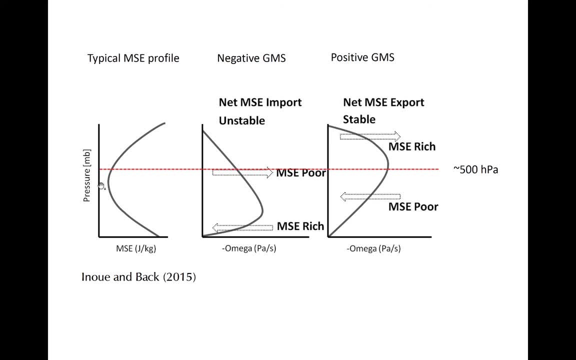 troposphere. Negative GMS occurs when the net transport of MSE into a column is positive. The middle panel shows an example of convergence in the low troposphere and divergence in the middle troposphere, where MSE is low. Comparatively, the MSE is high in the low troposphere. This might occur in an environment. 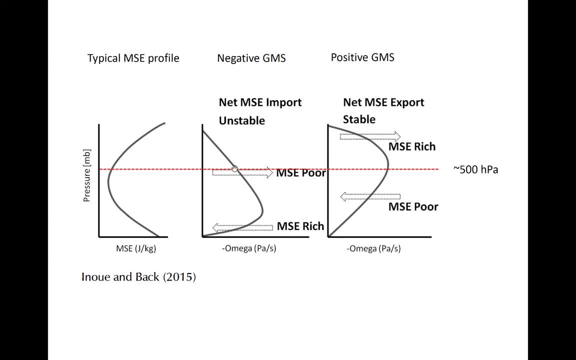 with a low-level maximum in vertical motion, such as when shallow convection is present. That's what this gray line represents is a hypothetical omega profile. In this case, the column-integrated divergence of MSE would be negative. In other words, there would be net convergence of MSE in the column, making it more unstable. 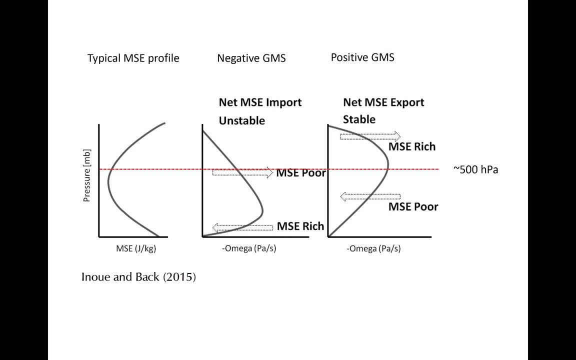 The right-most panel shows a contrasting example of a vertical motion profile that we would call top-heavy. It has an upper tropospheric maximum which is more indicative of deep convection. In this case, convergence occurs through a deep layer in the low-to-middle troposphere. 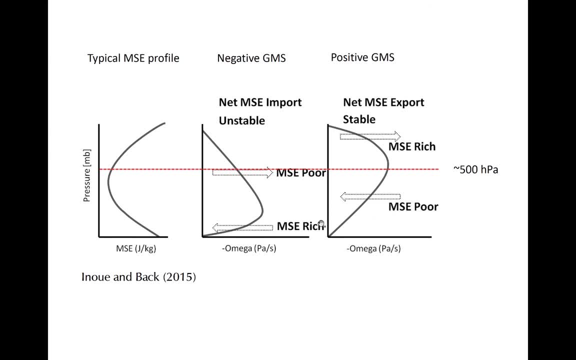 so the net convergence of MSE into the column is lower than in the first example. Divergence occurs in the upper troposphere, where MSE is large. Therefore, net divergence of MSE in the column is positive in this example, meaning that convection stabilizes the environment. It does so by transporting MSE from the boundary layer. 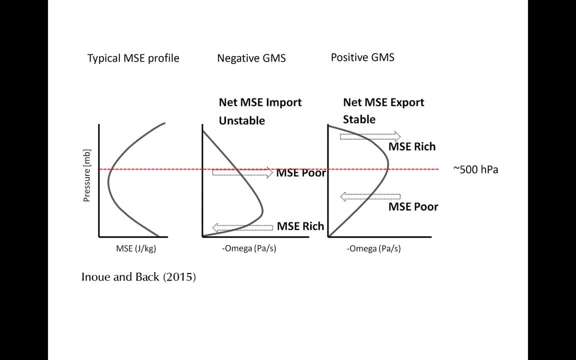 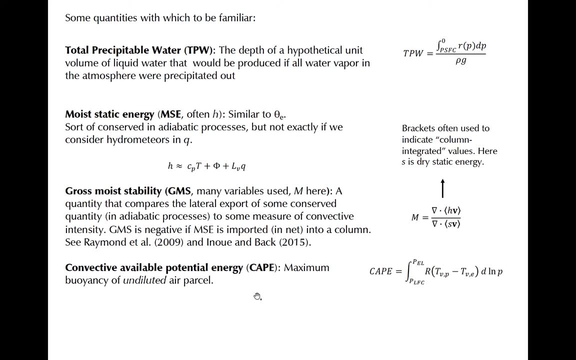 to the free troposphere. Finally, convective available potential energy, or CAPE, is a useful metric to consider when consulting soundings. It is proportional to the difference in parcel and environment virtual temperatures integrated from the level of free convection to the equilibrium. 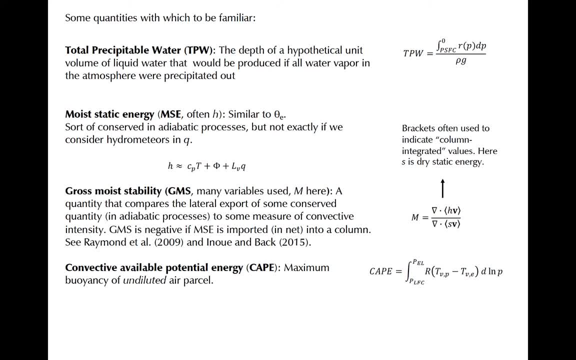 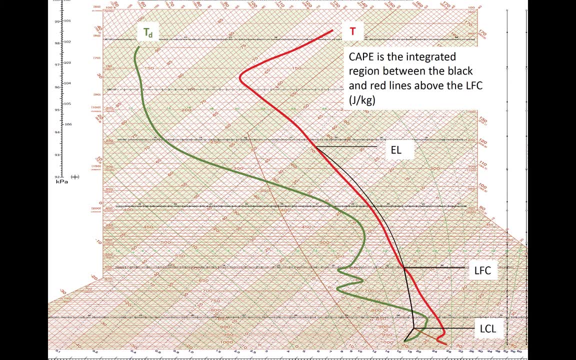 level which we will define on this QT plot in a little bit Back to our example sounding from the last module. if we look at this particular example, the CAPE is the region between the black line and the red line above the LFC. How exactly the CAPE is calculated? 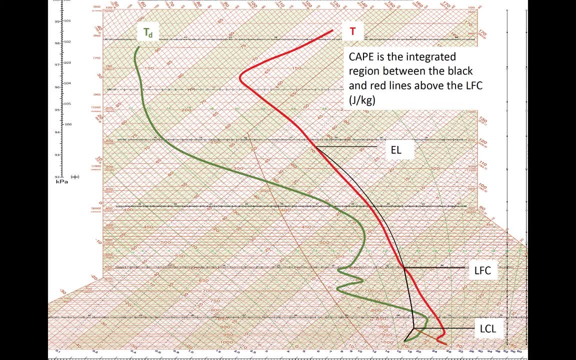 depends on exactly how the moist layer is treated and what the depth of the moist layer is and some other assumptions. But in this example I've represented surface-based CAPE. That means that I connect a dry adiabat and a line of constant mixing ratio as if I were computing theta E. 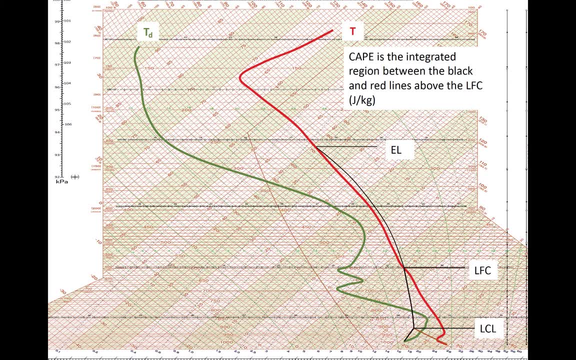 then follow it up the moist adiabat until it reaches the equilibrium level, which is the level above the LFC where the parcel temperature has cooled to the environmental temperature. So if I'm starting at surface temperature and surface dew point, follow this. 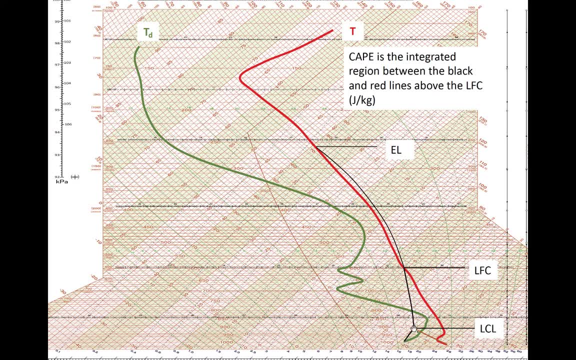 dry adiabat until it intersects this mixing ratio line and follow the moist adiabat up The integral of the space between the black line and the red line in this area. here is your CAPE. This particular sounding has very little CAPE, primarily because the boundary layer is fairly 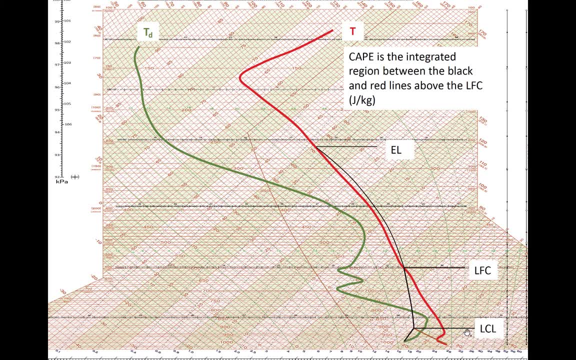 dry, The LCL, the L-ice, the L-y-c-e-o-l-r. The lifting condensation level is the pressure level at which the dry adiabat, representing the initial boundary layer parcel, meets the mixing ratio line represented right here. 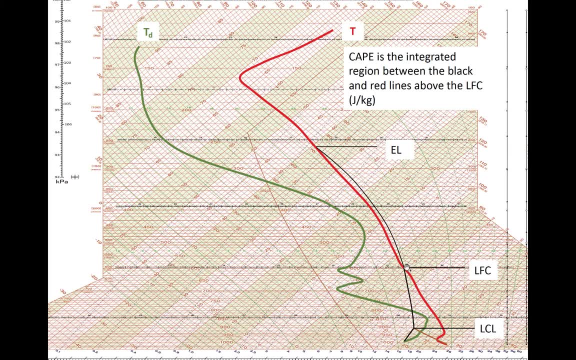 The LFC is the pressure level at which the parcel is no longer cooler than the environment as it rises. So this black line would be the hypothetical parcel temperature compared to the red line, which is the environmental temperature. When I say hypothetical parcel temperature, I'm talking about a parcel that's lifted. 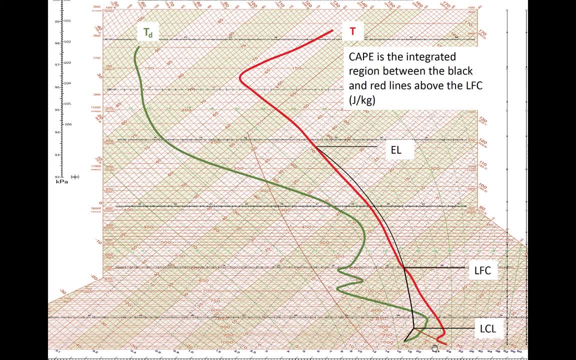 from the surface. with this humidity- excuse me this dew point- and this temperature, If I were to add some moisture to the boundary layer, you can clearly see the impact on CAPE. Suppose the blue line down here toward the bottom instead of the green line represents. 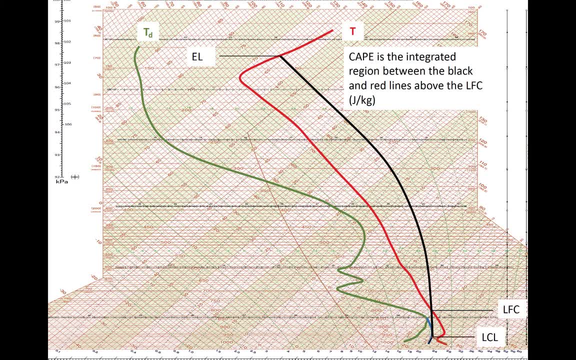 the dew point below 850 millibars. In this case, the surface-based LCL is around 970 millibars, Which is actually quite low. The LFC is around 800 millibars and the equilibrium level is 140 millibars. 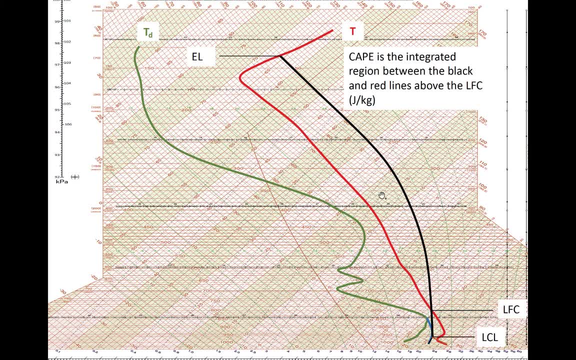 This sounding has much more CAPE, meaning that an undiluted updraft that reaches the LFC could become particularly intense. So this region right here represents the CAPE in this sounding. This shows how moisture is not only important to convection, because updrafts can entrain 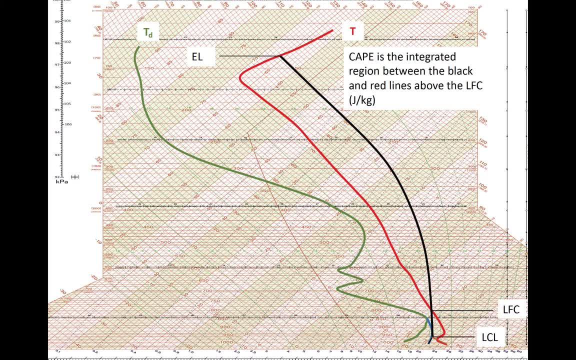 dry environmental air as they rise through the troposphere. This shows how moisture is not only important to convection, because updrafts can entrain dry environmental air as they rise through the troposphere. This shows how moisture is not only important to convection, because updrafts can entrain dry environmental air as they rise through the troposphere. 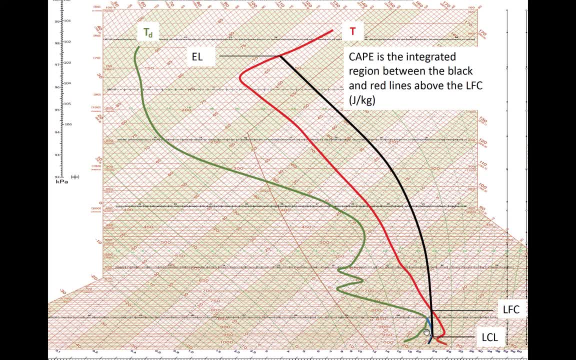 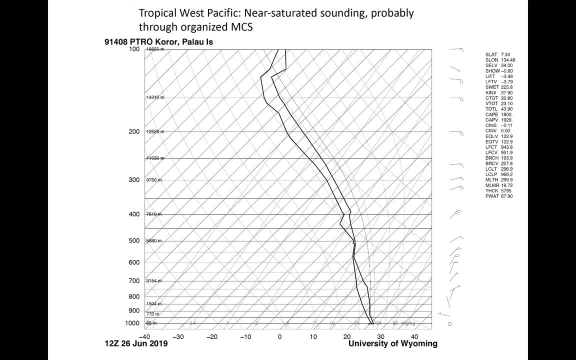 But also that the moisture content of the boundary layer directly impacts the convective instability of the environment. Let's look at a few examples of real soundings. In each sounding, the right most thick black line represents the temperature and the thinner black line to the right of that represents a moist adiabat that a parcel would follow. 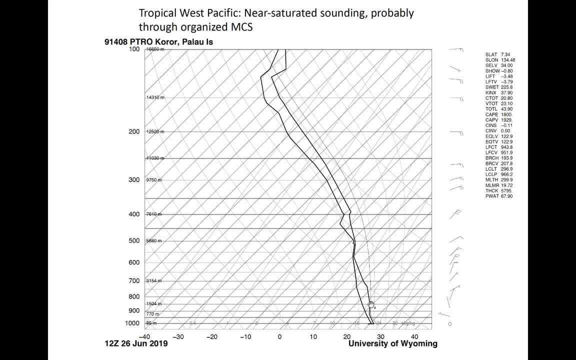 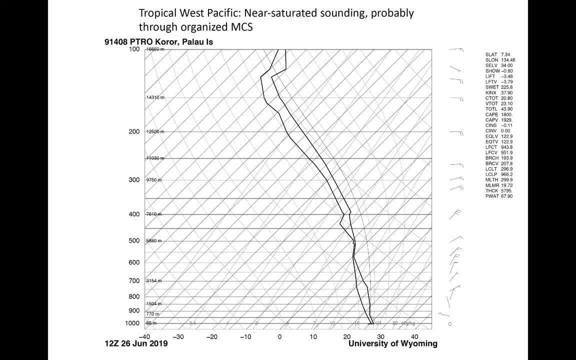 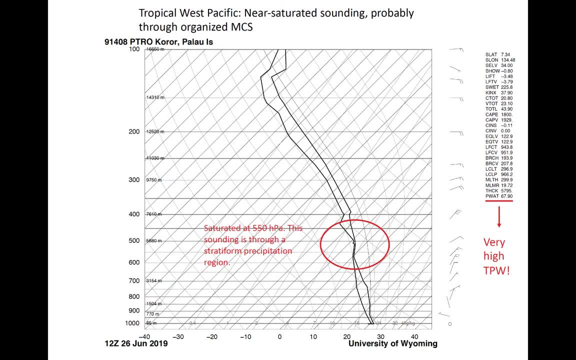 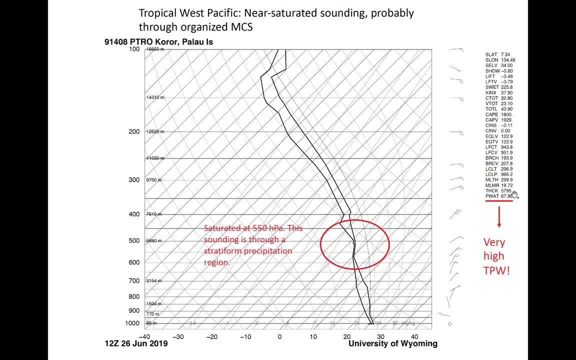 This is the adiabat. This is the adiabat. This is the adiabat was a very juicy 67.9 millimeters. The sounding mostly follows a moist adiabat but is conditionally unstable between roughly 750 and 600 millibars. so the CAPE was about 1,800 joules per kilogram. 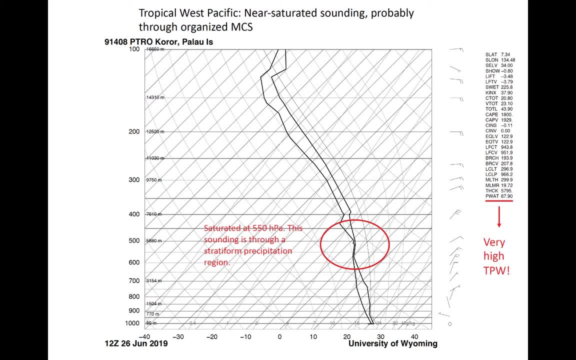 Although there is no set rule of thumb, CAPE over 2,000 joules per kilogram over tropical oceans is plenty sufficient to support deep convection, provided that sufficient moisture is present. This is in contrast with CAPE values over continental regions that can sometimes 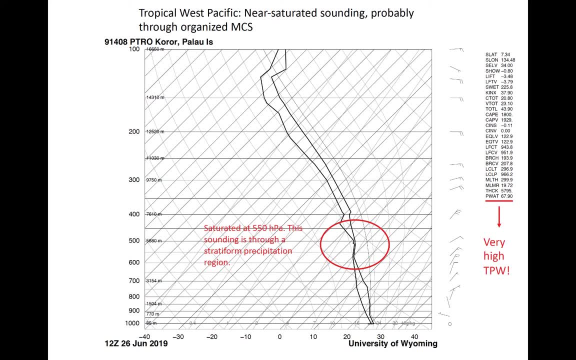 exceed 4,000 joules per kilogram during severe weather outbreaks. Such CAPE values are extremely rare over tropical oceans. In this case, the CAPE is distributed through a very deep layer in the troposphere, meaning that it will support updraft velocities much less than what you. 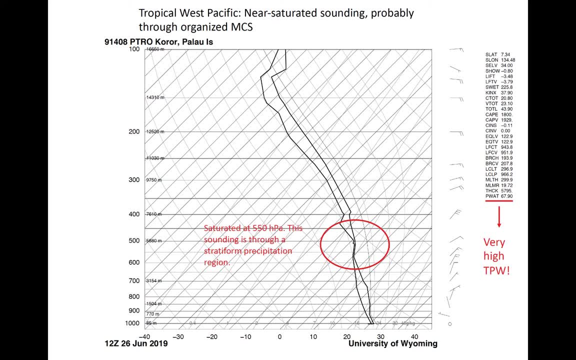 might see in continental convection. Typically speaking, marine convection is less intense than continental convection, The latter of which produces the majority of lightning globally. The sounding here is also saturated, close to the zero degree C level. If I saw this sounding with no additional context, I would assume it was launched into a stratiform precipitation. 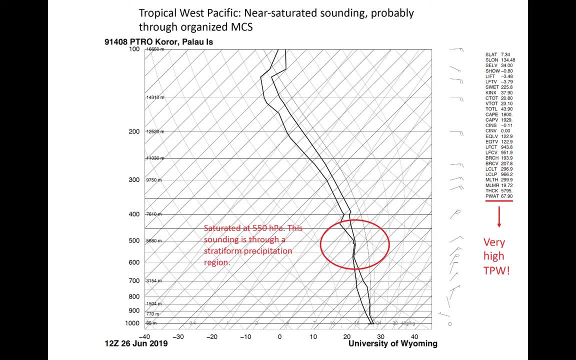 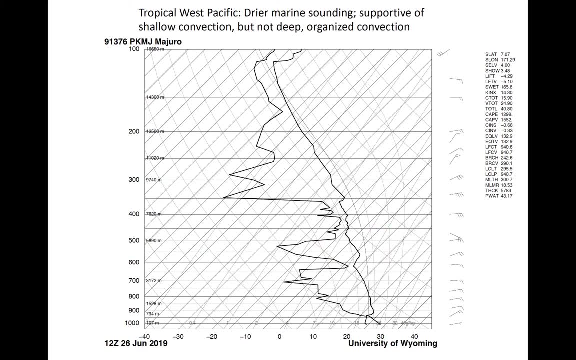 region in a mesoscale convective system. Depending on the situation, I might expect subsequent soundings to be more stable. This sounding is also from the tropical West Pacific, but it's much drier. Note that the TPW is much lower than before: 43 mm is a moderately low value for a TPW. 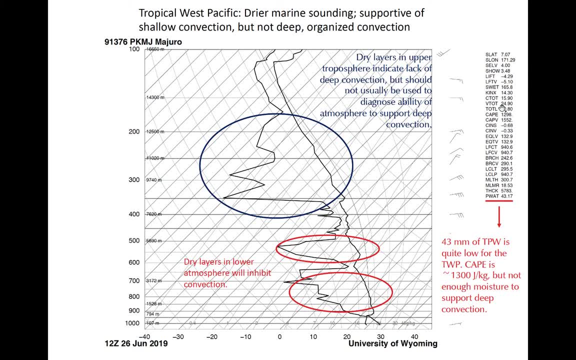 The CAPE in this sounding was estimated to be about 1,300 joules per kilogram. Thus the environment is buoyant enough to support vertical growth of an undilute parcel. However, this sounding indicates several dry layers. Two dry layers are seen in the lower troposphere. 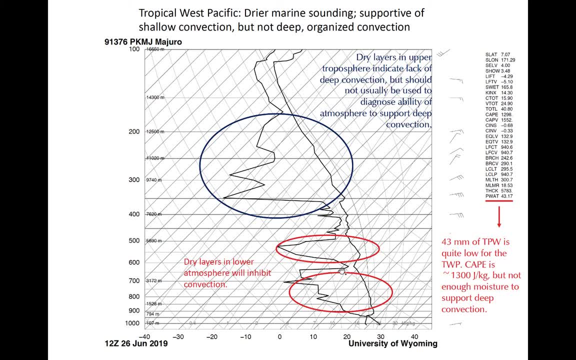 consistent with a low TPW reported. The dry layers are visible in the lower troposphere. These dry layers probably help reduce the energy level closer to the top than they show elsewhere. As for the dry layers that are seen in the low, These dry layers prevent widespread growth of convection because updrafts entrain the air. 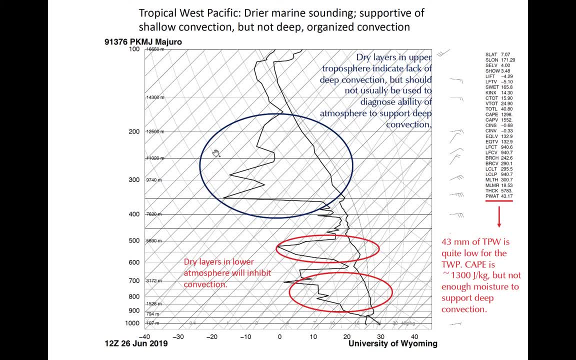 and become less buoyant. You'll also note that the upper troposphere is very dry. This is more indicative of the fact that deep convection is not present than it is of an environment unfavorable for convection. Cold upper tropospheric air can hold only limited. 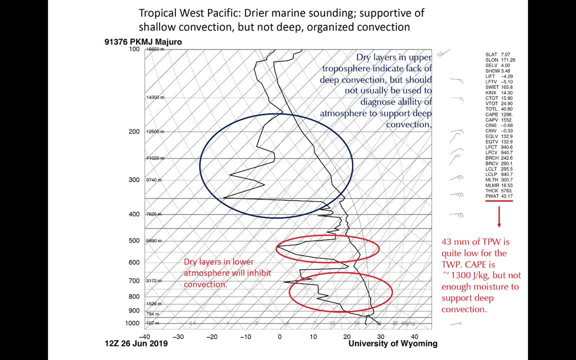 water vapor before reaching saturation, meaning that the difference between water vapor and cloudy versus environmental air in the upper troposphere is generally small. A corollary to this is that the common relative humidity on which rainfall depends on is most heavily influenced by the humidity in the lower troposphere. 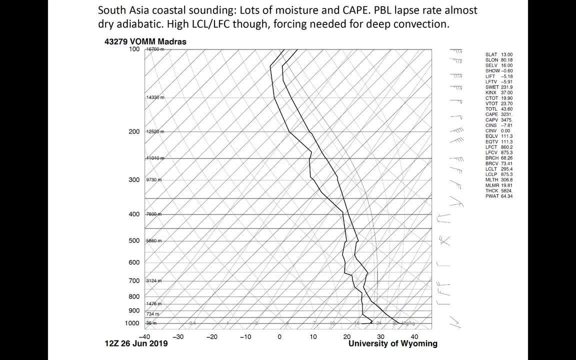 Next, here is a coastal sounding from South Asia, Madras, India. This is also very moist sounding, as seen by the TPW: over 64 millimeters. The difference here is that the temperature profile of the boundary layer points to a low temperature profile of the boundary layer. 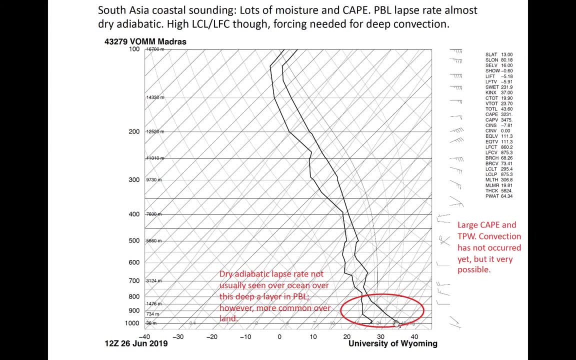 This is a quite unstable sounding. Usually, environmental lapse rates are much less than the dry adiabatic lapse rate over well-mixed marine boundary layers, whose temperatures are controlled more by the underlying SST. Over land, however, boundary layer temperature is often less constrained and more impacted by insulation. 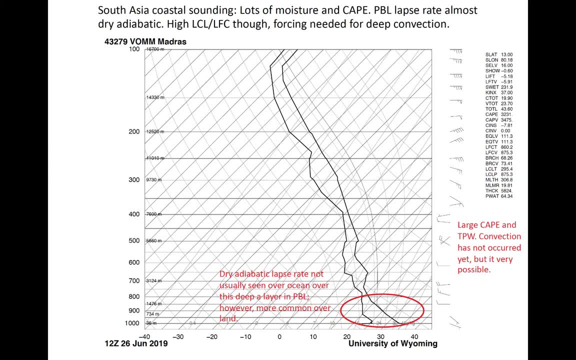 When this sounding was made, convection had not yet occurred near the station. However, a warm, moist boundary layer and steep lapse rate below 850 millibars certainly support deep convection. Note that the CAPE was over 3200 joules per kilogram. 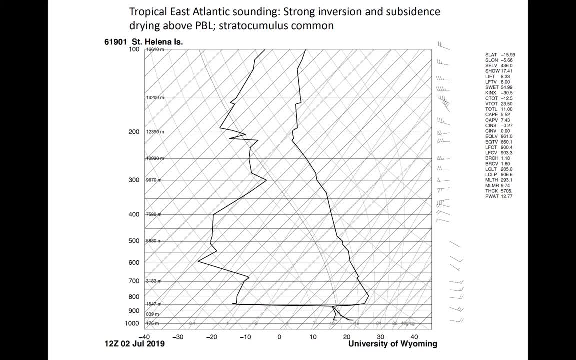 The next sounding is also in the tropics, but it looks very different. This one was taken from the tropical East Atlantic, in a regime with strong subsidence and where stratocumulus clouds are often quite common. The previous soundings were over regions of 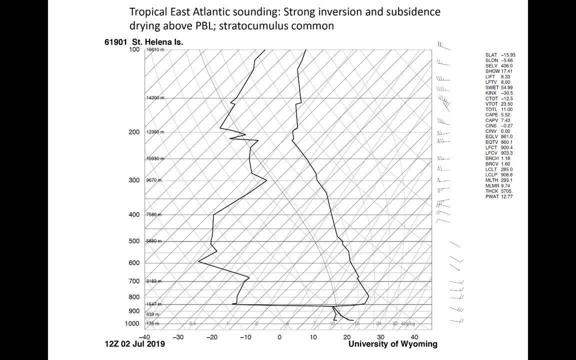 the Indo-Pacific Tropical Warm Pool. However, this one was taken over an island in a local location where SSTs are typically cool. Note the surface temperature in this sounding, which is a little under 20 degrees C. At about 850 millibars the temperature increases sharply and the dew point drops off very sharply. 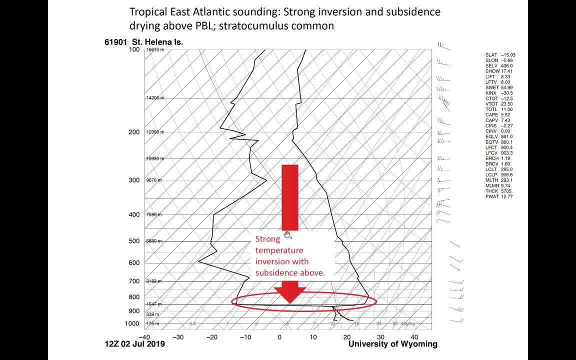 This is indicative of the bottom of a strong, deep layer of subsidence. Temperature increasing with height is called an inversion. Inversions indicate stability. They are often accompanied by dry layers that are indicative of descent. This sounding is not supportive of deep convection whatsoever. CAPE is basically zero and the 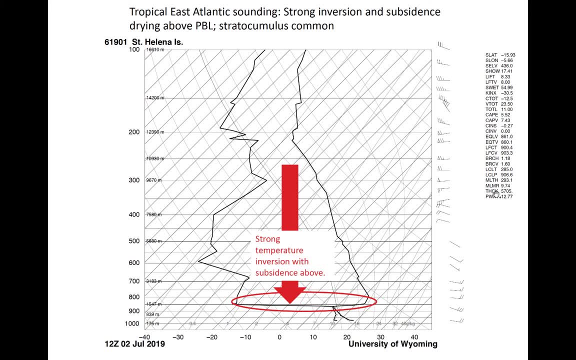 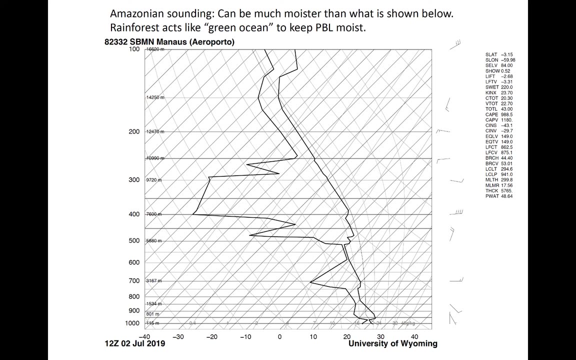 TPW is restricted by the inability for deep convection to form and transport water upward. However, as I said before, boundary layer stratocumulus can form and persist. in an environment with a sounding like this. The Amazonian rainforest can behave like a green ocean in terms of service. 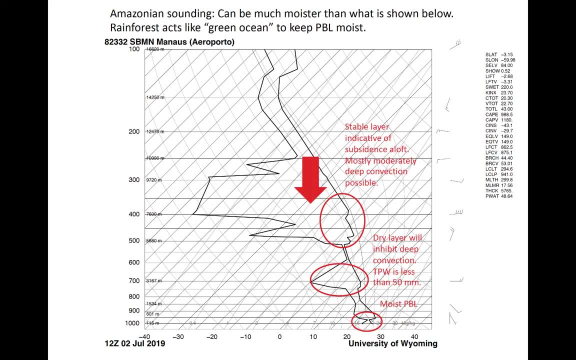 fluxes, fluxes. This sounding features a moist planetary boundary layer and above 1,000 joules per kilogram, or about 1,000 joules per kilogram in CAPE, but it contains a dry layer centered near 700 millibars that will inhibit convection. 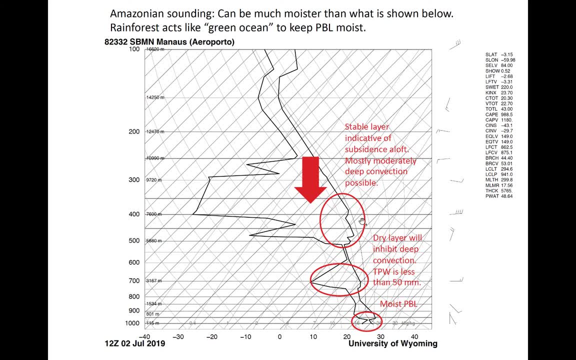 The stable dry layer above 500 millibars indicates subsidence. again, It's possible that this thermodynamic profile could support some shallow and moderately deep convection rooted in the boundary layer. but deep convection will struggle to survive for long periods of time. 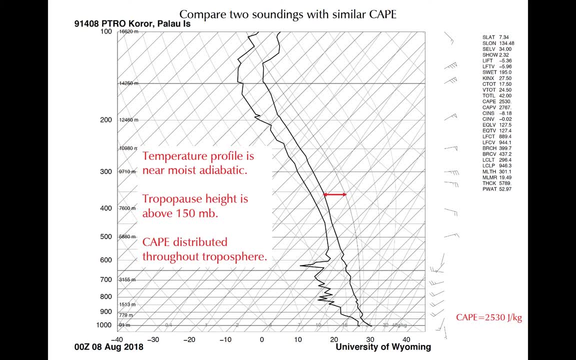 Finally, we will end with a word of caution about using just CAPE to assess the likelihood of strong convection. We've already mentioned that the CAPE needed over tropical oceans to support widespread rainfall is much less than that often seen over continental regions during outbreaks. 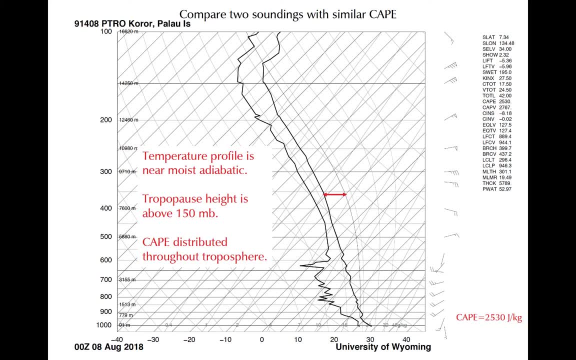 of deep convection, such as over the central US in springtime. We will next compare a couple of marine tropical soundings with continental soundings. Here we are looking at a sounding from Palau, with a temperature profile that is nearly moist, adiabatic. 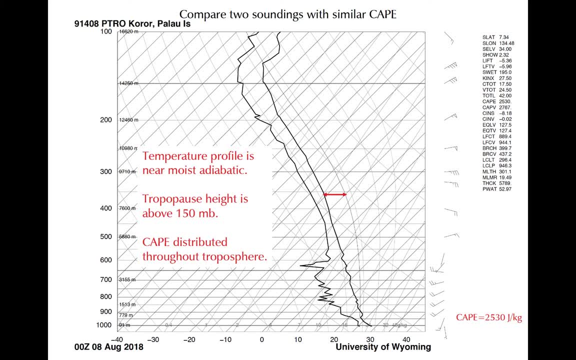 The CAPE, like before, is distributed through the troposphere in a deep layer. Total CAPE is about 2,500 joules per kilogram. however, the lower free troposphere is not particularly moist, between 900 and 600 millibars, where it is conditionally unstable. so the 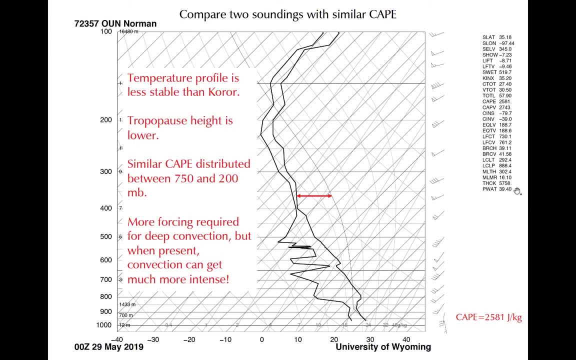 TPW is only about 53 millimeters. The lower free troposphere is not particularly moist, between 900 and 600 millibars, where it is conditionally unstable. so the TPW is only about 53 millimeters. Next look at a springtime sounding from Norman Oklahoma. 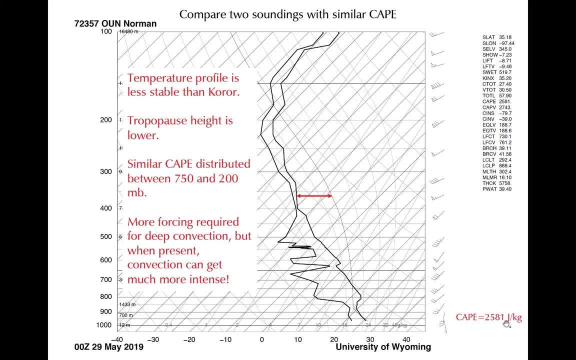 The CAPE is virtually the same as the Palau sounding. however, the lapse rate in the middle troposphere is steeper and the CAPE is concentrated more in the middle to upper troposphere than it is broadly distributed through the troposphere. In this example, more forcing is required so that convection can reach its LFC. however,